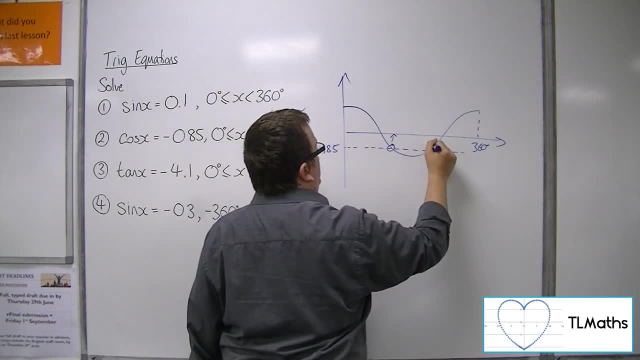 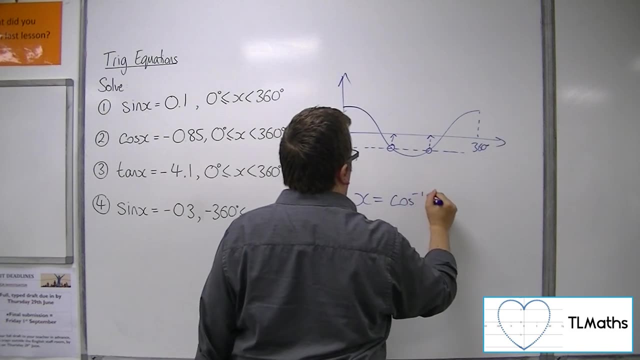 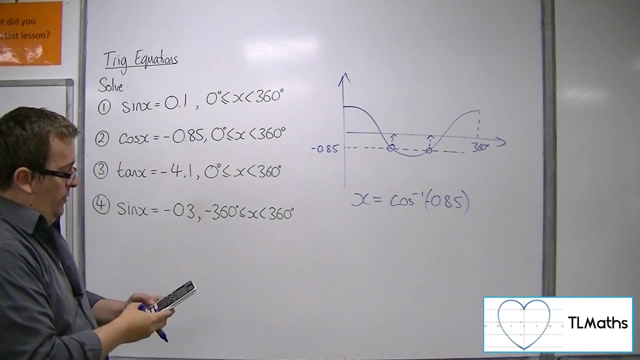 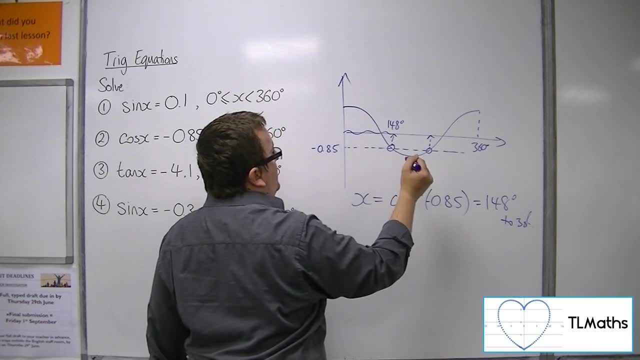 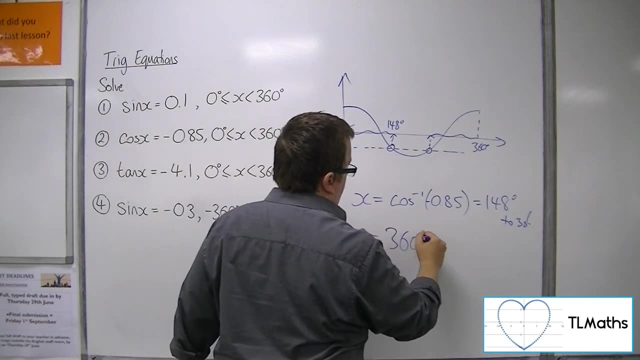 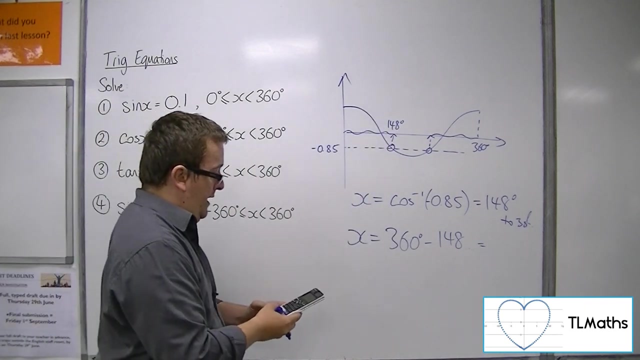 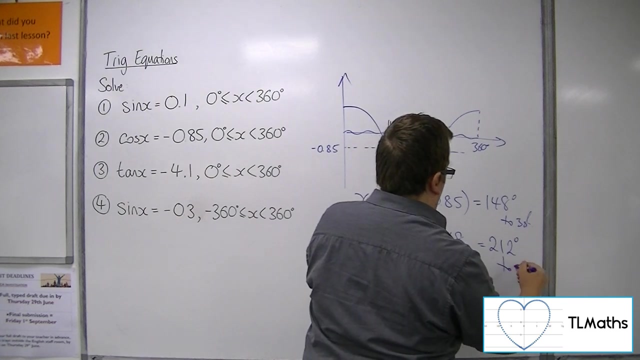 Now, that is 148 degrees. So this must be 148 degrees away from the 360. So 360, take away the 148. Okay. Use the full calculator display that you've still got in your calculator. 360, take away the answer key, is 212 degrees to three sig fig. 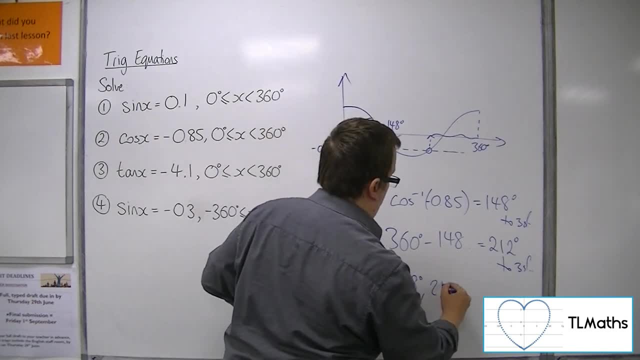 So... x has two solutions between 0 and 360. Okay, so that's number 2. 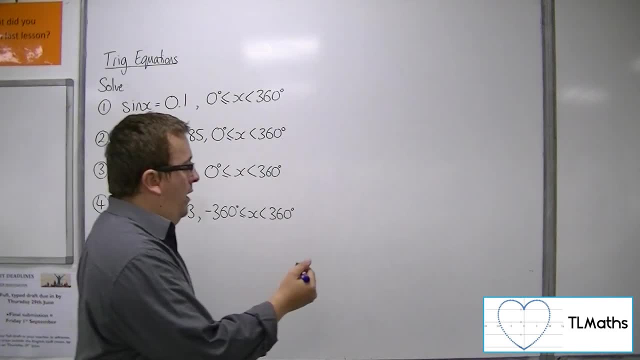 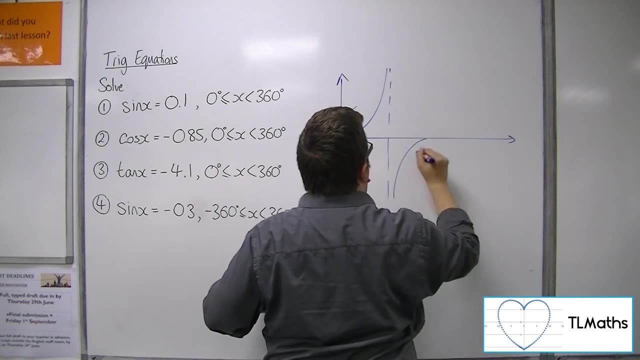 Now, number 3, tan x is minus 4.1. So, a sketch of tan, okay, so there's 360, there's 180. 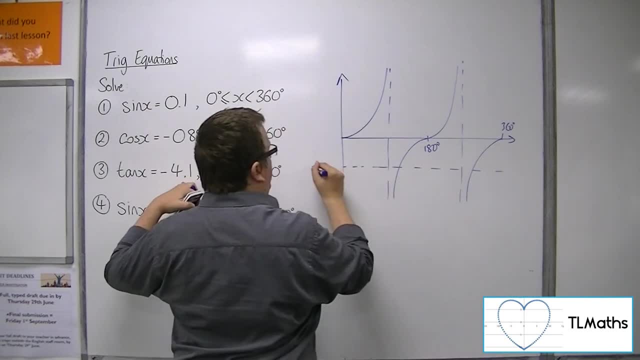 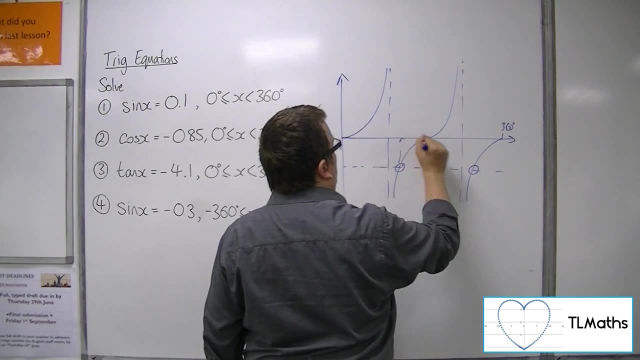 Now, minus 4.1, somewhere down there, okay. Now, there are two solutions that we can see between 0 and 360, okay. 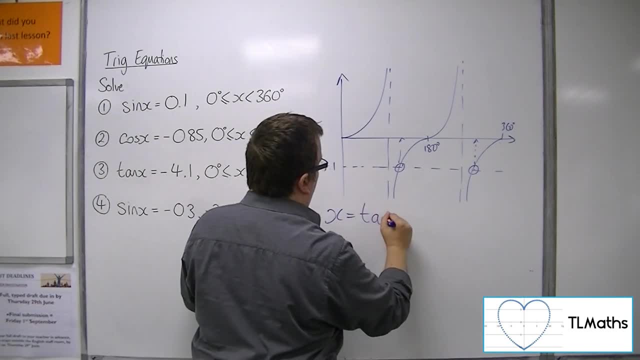 Now, if you do inverse tan. Of minus 4.1. Minus 4.1. 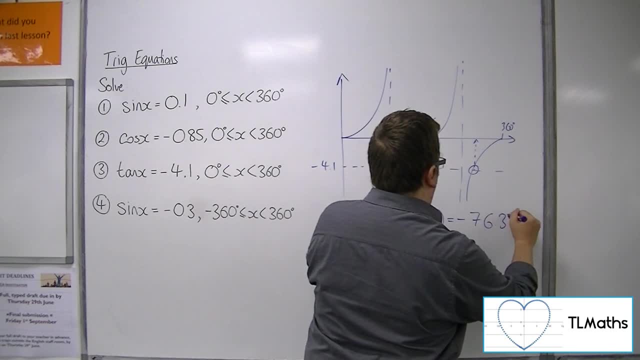 You get minus 76.3 degrees to three significant figures. 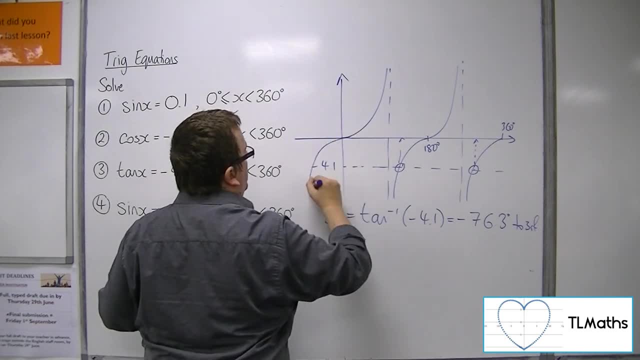 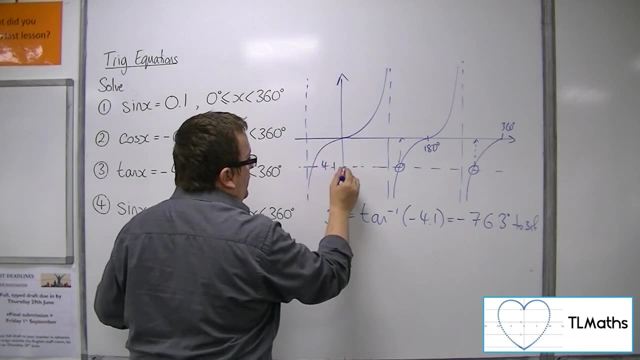 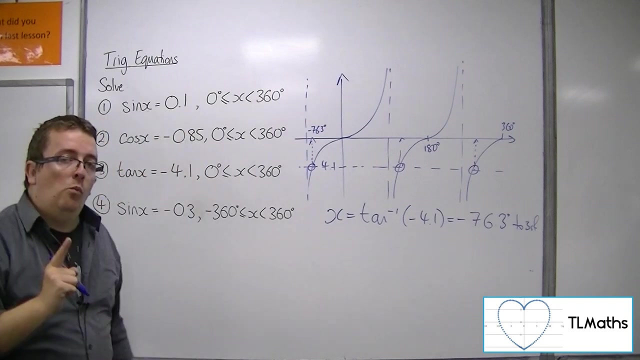 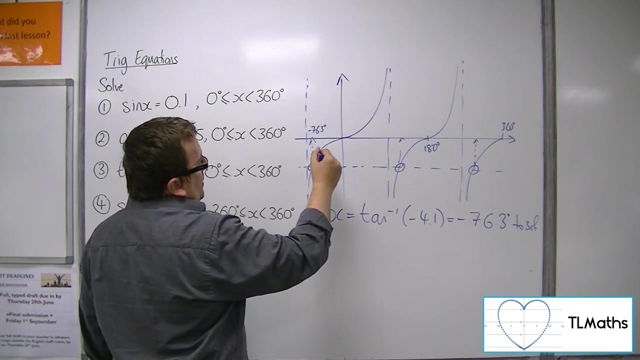 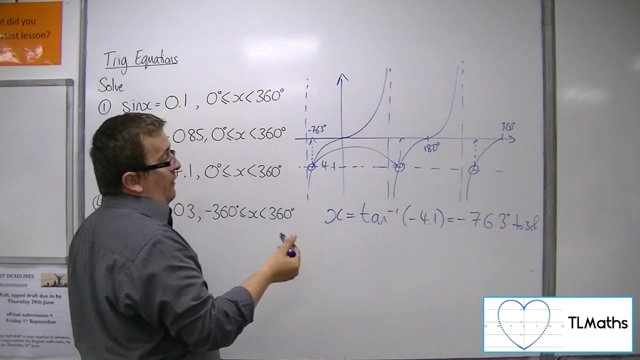 Now, what's happening is this, okay. The curve, okay, as we know, continues to the left of the wax, just like this. And this is the solution you are finding. Okay, now it's not one of the solutions that you want, you want these two. Now, because tan has this period of pi, you can just add pi, oh, sorry, of 180. I should make sure of 180 degrees, okay. 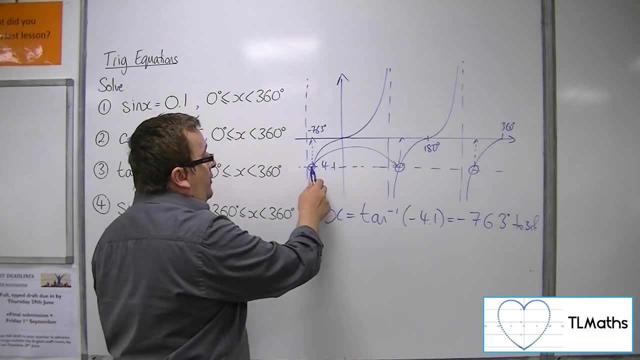 So, tan has this period of 180 degrees, and so you can just add tan on to get the next one and then the next one. 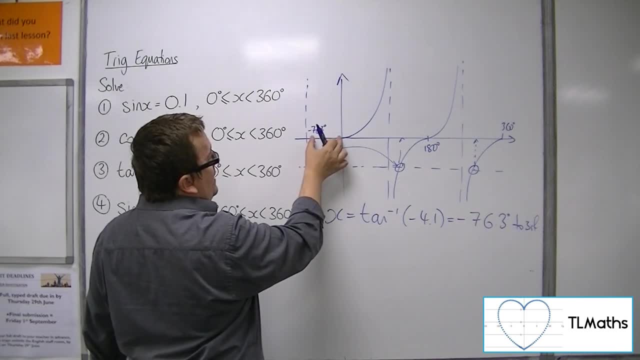 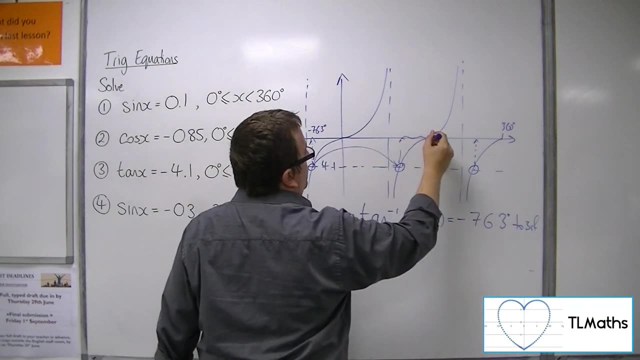 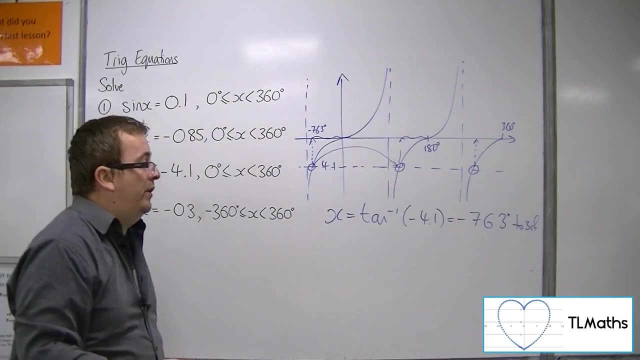 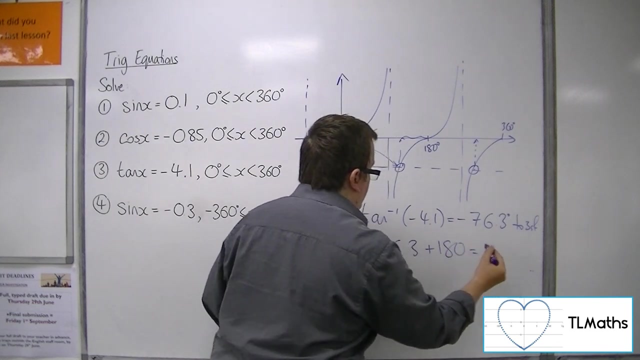 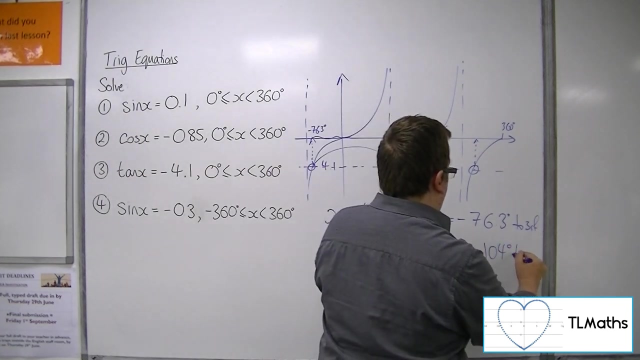 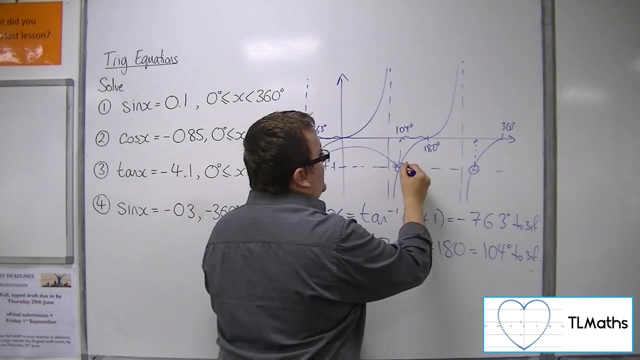 Now, you can visualize this by thinking, well, that is minus 76.3, or 76.3 in distance. And so, that must be 76.3 in distance as well. So, you can do 180 take away 76.3, if you want to think of it that way. Personally, I prefer to think of it as adding on 180, all right. So, add on 180, we get 140. So, that's the 104 degrees to three sig fig. Okay, so that's the 104 degrees, and then you can add on 180 again to get to the next one. 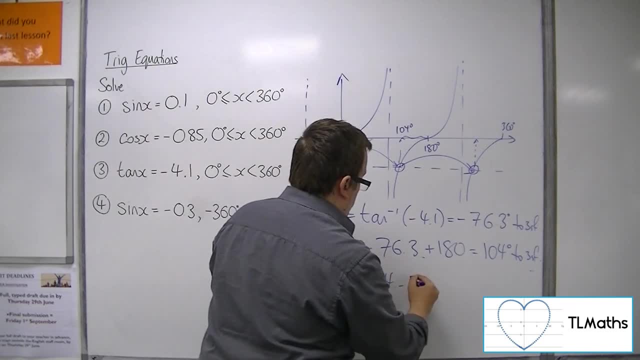 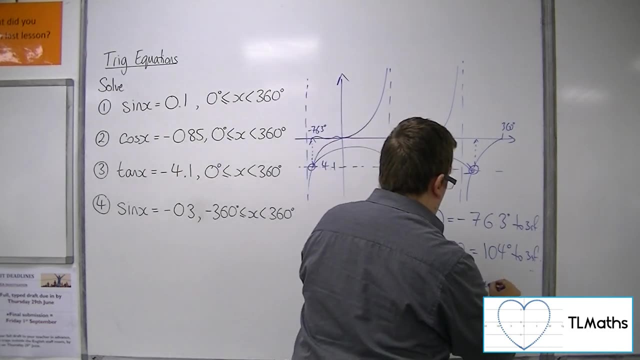 So, 104 plus 180, okay, gets us to 284 degrees to three sig fig. 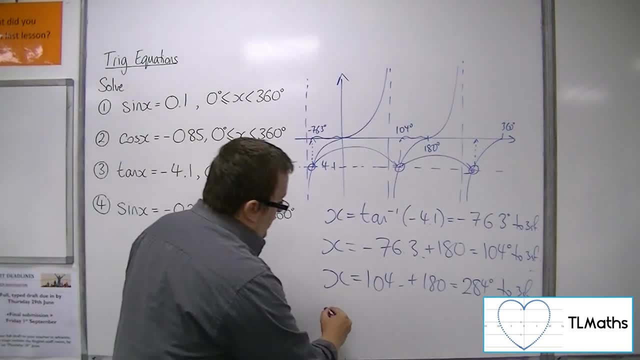 Now, you got to be careful to make sure that when you're saying, which are your sig fig, to be careful to make sure that when you're saying, which are your sig fig. 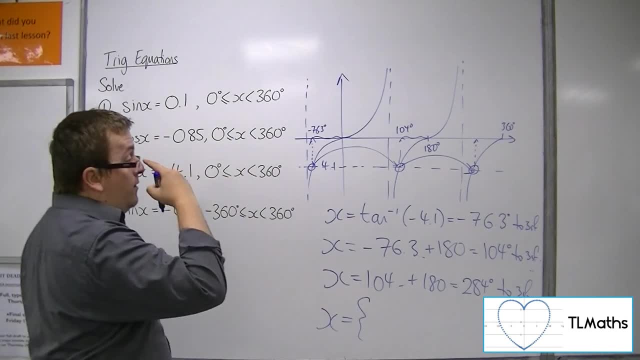 solutions that you pick the ones that are between 0 and 360 so we don't 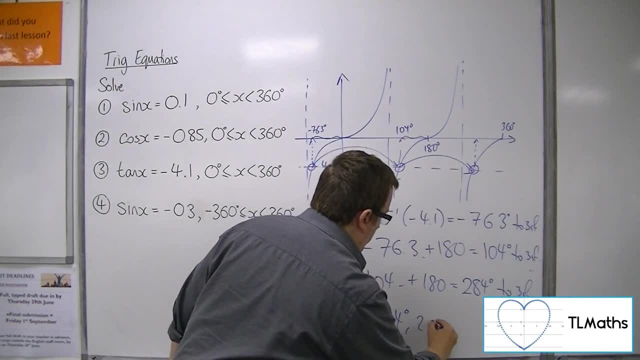 include that one we're just looking at 104 and 284 to 3 sig fig okay and that's 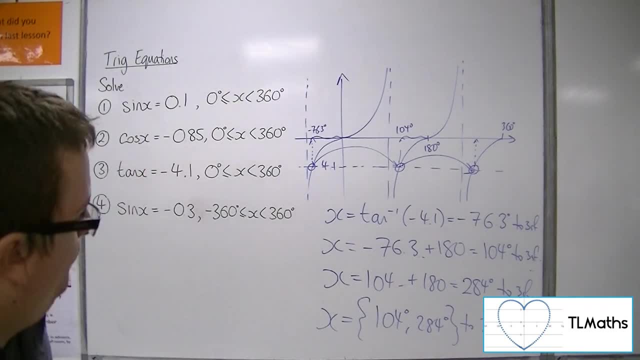 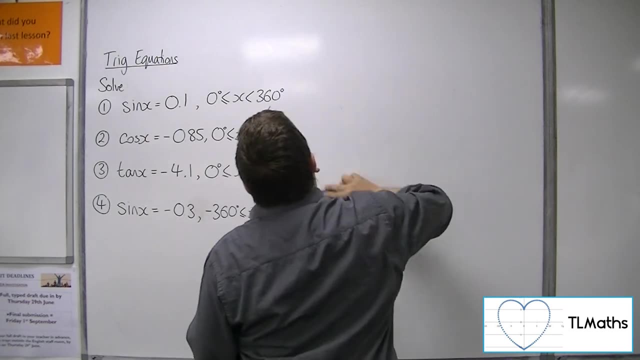 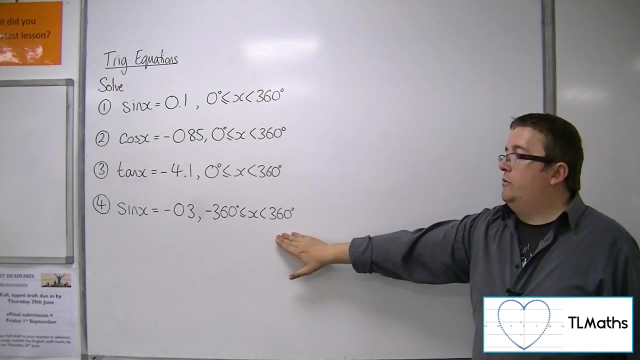 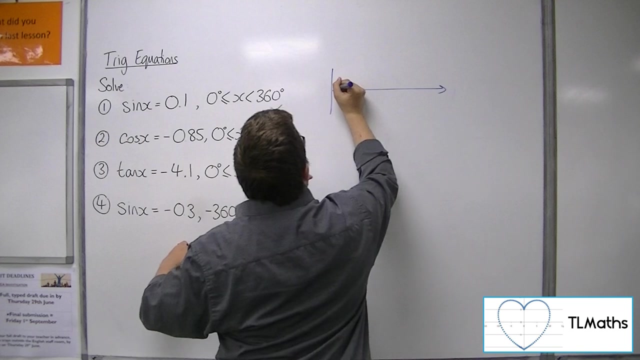 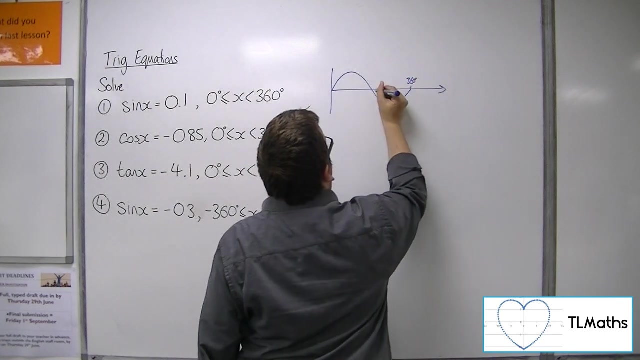 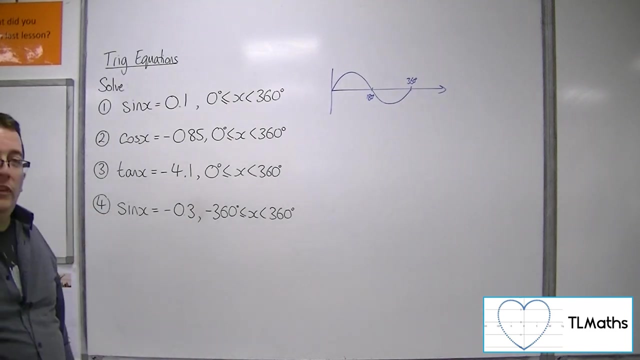 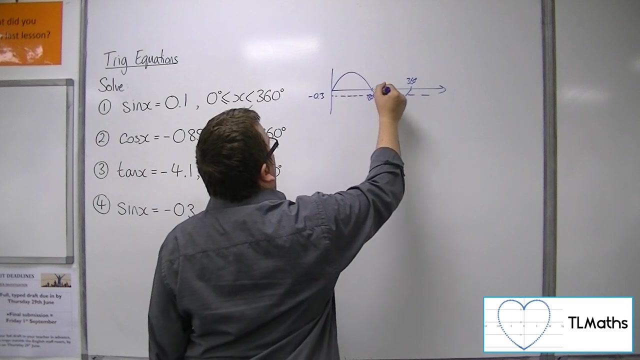 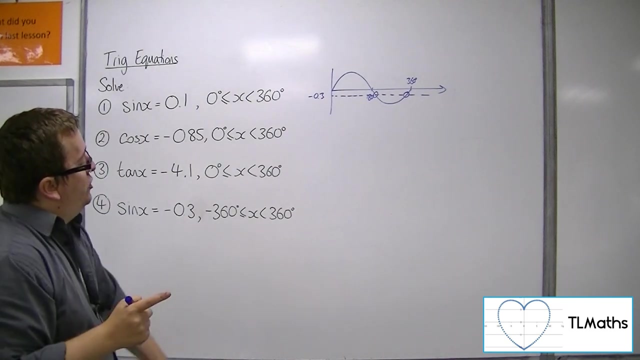 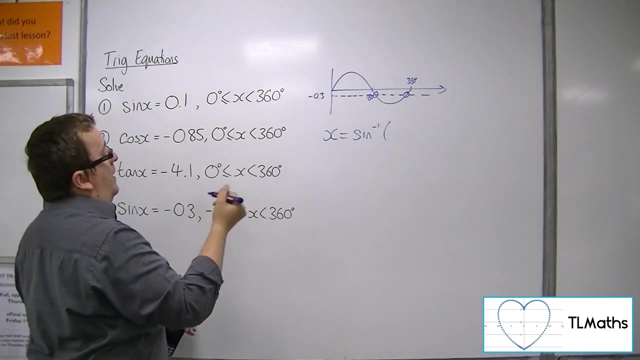 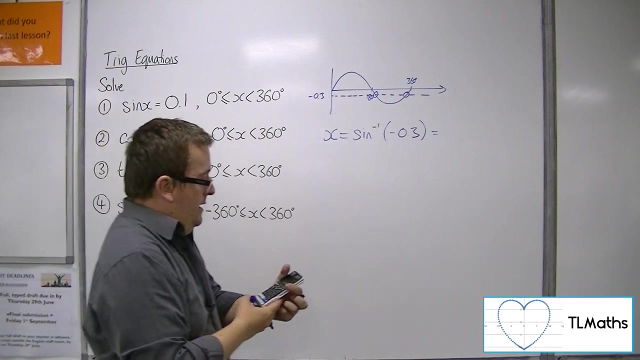 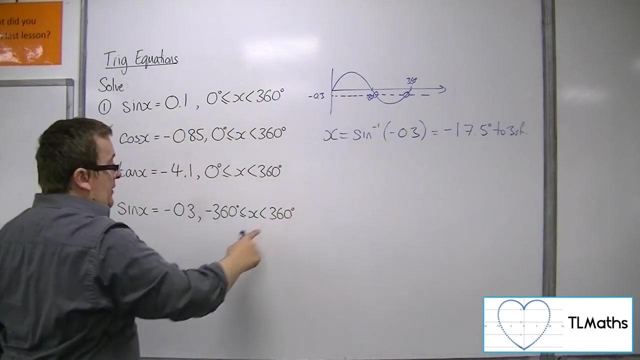 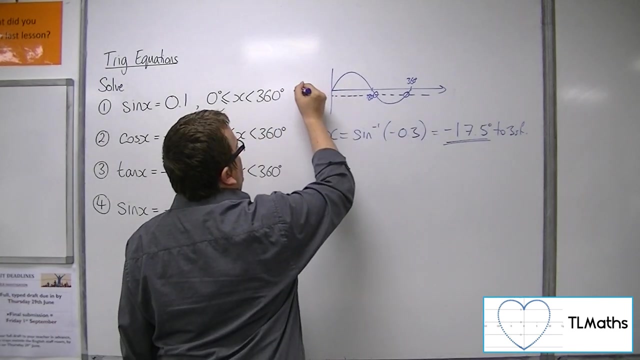 how we can solve number 3 right now the last one here okay I've put it as but being between minus 360 and 360 okay so I'm still only going to sketch sine between 0 and 360 okay I don't really worry about sketching one that is between minus 360 and 360 so minus naught point 3 will be a horizontal line and we can see that there are two solutions between the 0 and 360 that I want there I want the solutions between minus 360 and 360 so let's see what happens so inverse sine of minus naught point 3 so inverse sine of minus naught point 3 is minus 17.5 degrees to 3 sig fig now that is an answer between minus 360 and 360 so that is perfectly good as a solution now the reason why you're getting that solution is because the curve is continuing background right and your calculator is picking up that solution there. 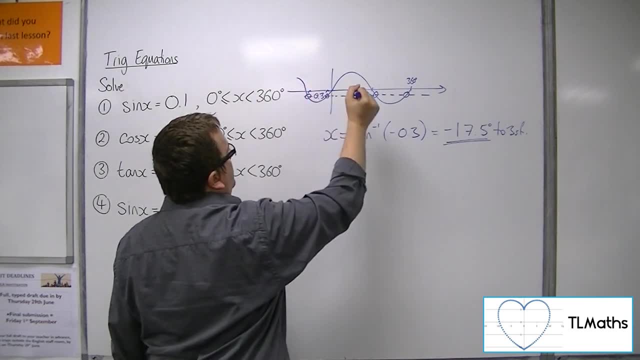 So the other solution will be there, and there's one there, and there's one there. 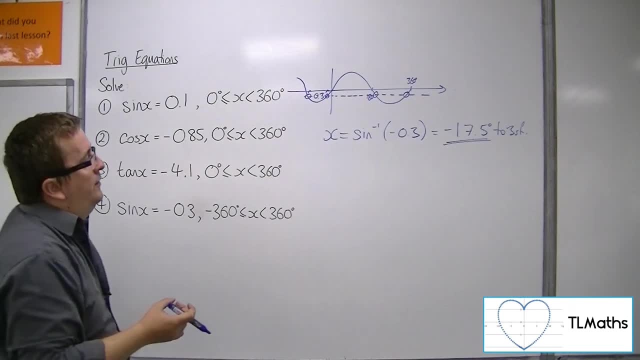 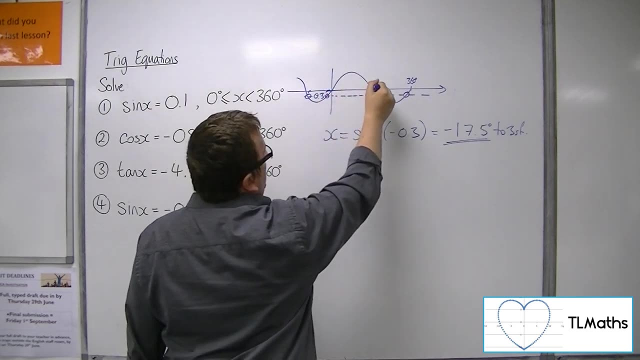 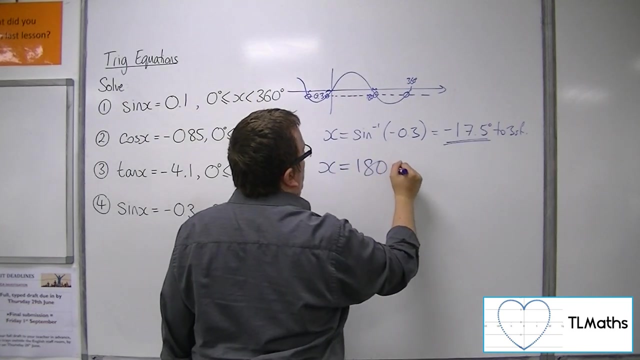 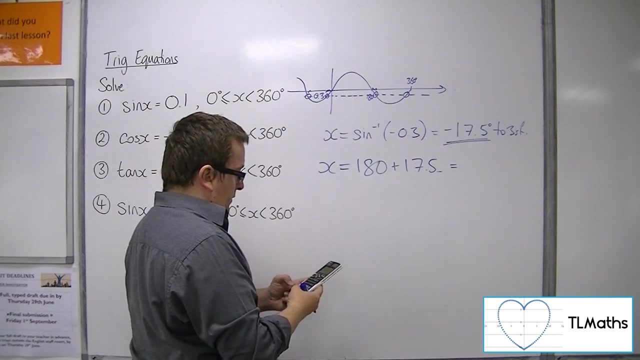 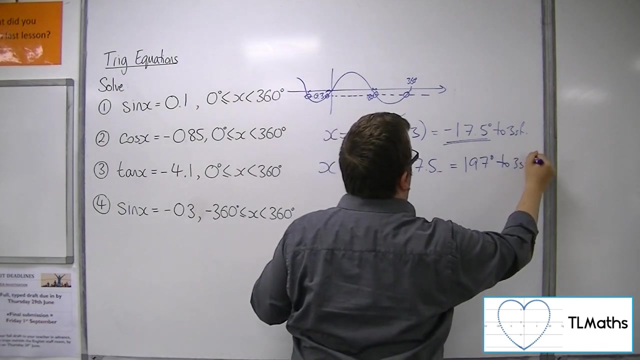 Now, minus 17.5 degrees is a perfectly valid solution. That means that that distance there is 17.5. So that distance there is also 17.5. So I can add 180 to the 17.5. So times by minus 1, add 180, and we get 197 degrees to three significant figures. Okay. 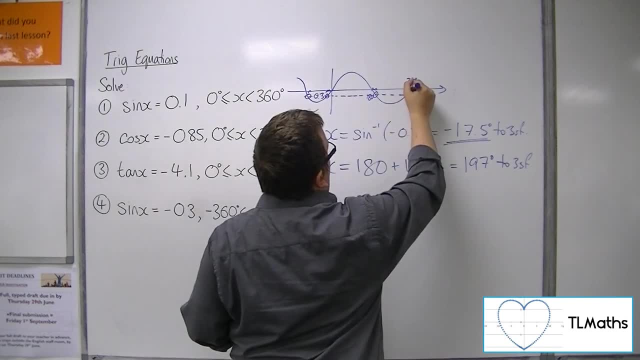 Then, if that's 197, that bit is also 17.5 degrees away from 3. So that gives me 360. Okay.